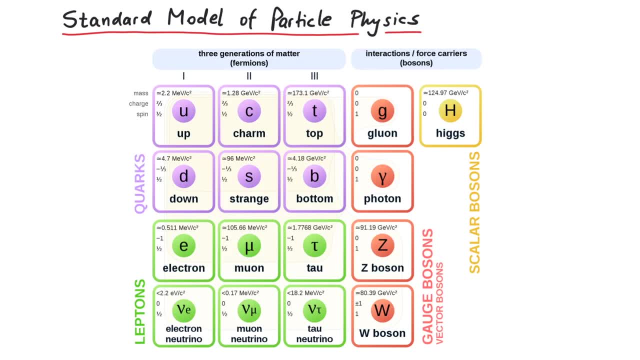 The standard model of particle physics contains two kinds of particles: fermions and bosons. All fermions have half integer spin and are again separated into two categories: quarks and leptons. Among those there are three categories, so-called generations. 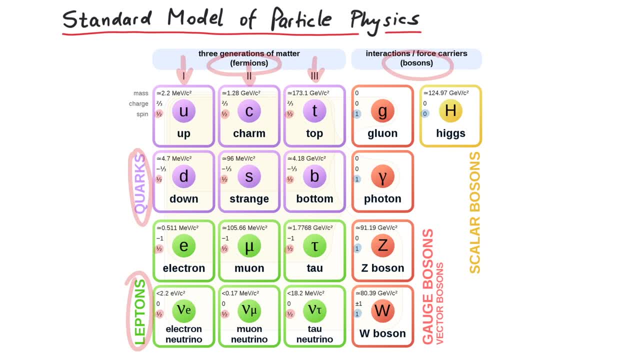 And for bosons, particles carrying integer spin, we can distinguish gauge bosons who mediate a force and the Higgs boson. In this video we will focus on leptons. The first generation of leptons contains the electron and the electron neutrino. 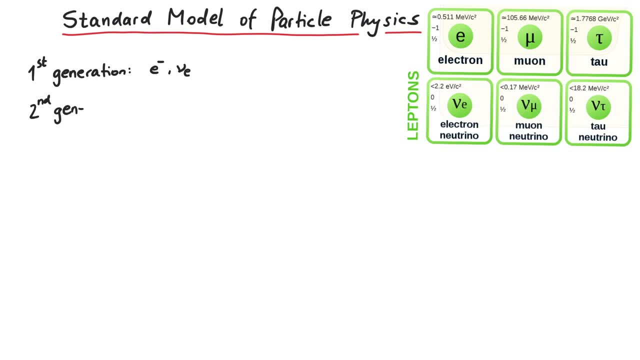 Higher generations have very similar properties, but higher mass. There we have the muon and the mu-neutrino, as well as the tau and the tau-neutrino. Every lepton also has an antiparticle, which is usually denoted with a plus or a bar on top. 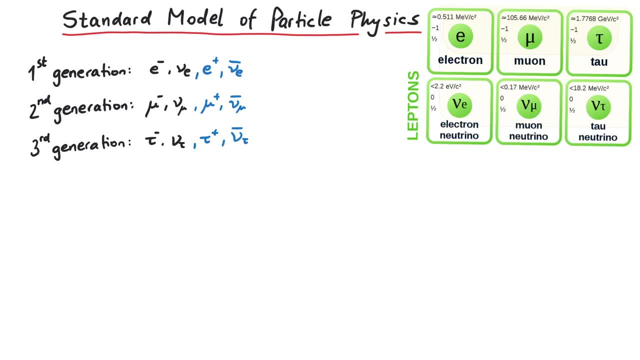 The antiparticles have the same mass but opposite charge. This refers to electric charge, but also to a quantity called lepton number, which is the main thing. Lepton number is defined such that leptons are assigned the value plus one and antileptons get the value minus one. There are actually three kinds of lepton numbers. 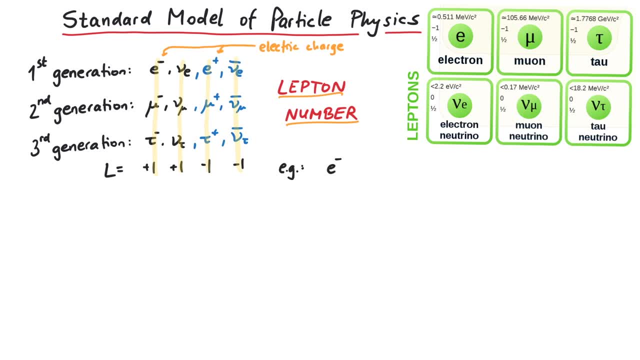 one for each generation or family. So an electron has electron lepton number plus one, but tau lepton number zero. An anti-mu neutrino has mu lepton number minus one and electron lepton number zero, The total lepton number. 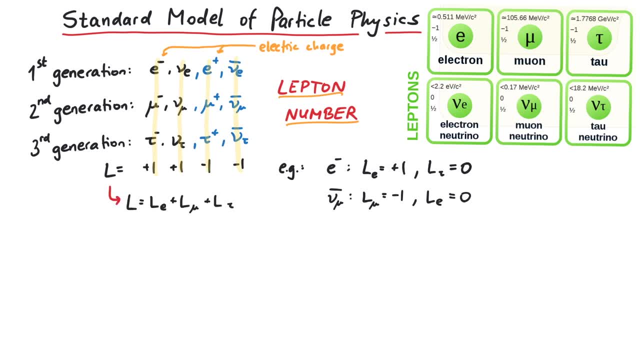 is then given as the sum of all other lepton numbers. In the standard model of particle physics, these lepton numbers are conserved when particles interact with each other. Let's look at two examples. First, let's consider radioactive beta decay. 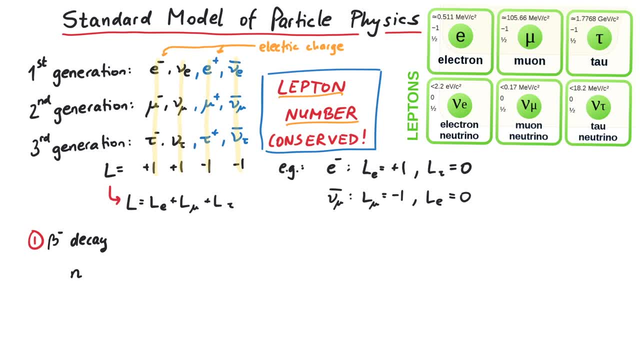 in particular beta minus decay. This describes how a neutron decays. The first decay product is a proton. It has positive charge, so we need some negative charge to balance it. So let's put an electron here. Electric charge is balanced. But what about lepton number On the left? 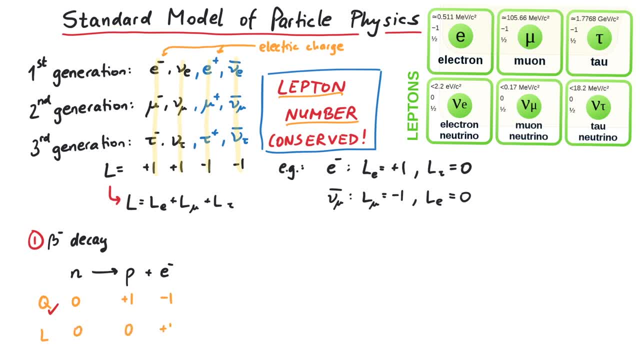 the lepton number is zero, but on the right the lepton number is plus one. Therefore we need an anti-lepton, in particular, either a positron or an electron anti-neutrino, Since the positron would disturb the charge balance, again we have to choose the electron. 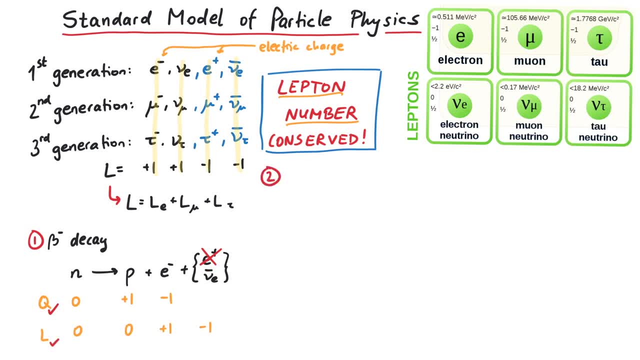 anti-neutrino. For our second example, let's consider the muon decay. If we look at this process very detailed, the muon first sends out a w-bar and then sends out a muon decay. The muon decays out a W boson and this W boson decays further into a lepton. 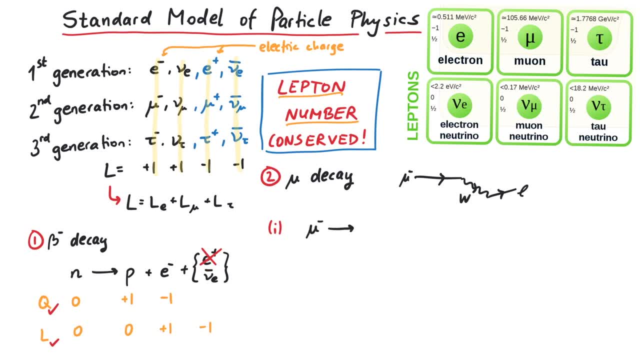 The first part of the reaction is therefore: muon decays into W boson. For electric charge conservation, we need to negatively charge W boson. And for lepton number conservation, Well, on the left-hand side we have mu lepton number plus one. therefore, we need either a muon or a mu neutrino on the right. 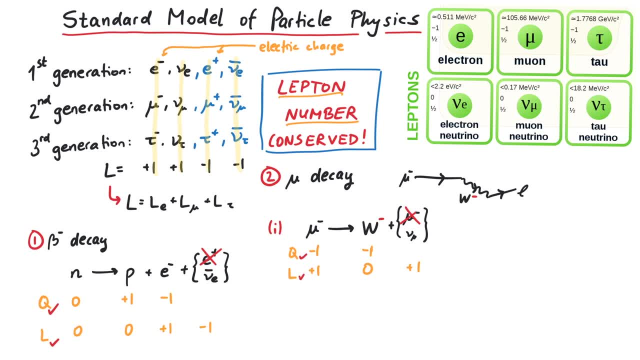 side, Due to electric charge balance, we choose the neutrino And for the second part the negative. If W boson decays into a lepton, usually it's the lightest one. so either an electron or a positron. Again due to electric charge balance, we have to choose the negatively charged electron. 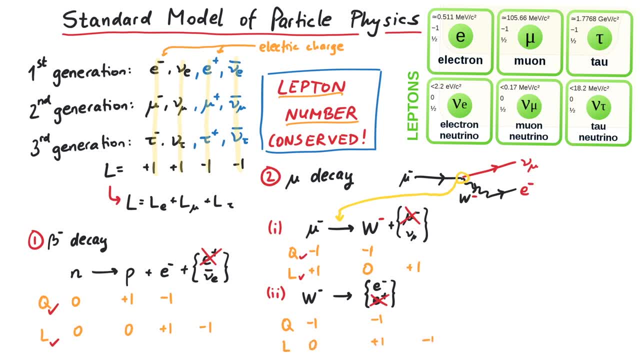 But in order to account for lepton number conservation we also need an antineutrino. here The correct choice is an electron antineutrino. Well, actually, the conservation law for the three lepton numbers separately is only valid for massless neutrinos.